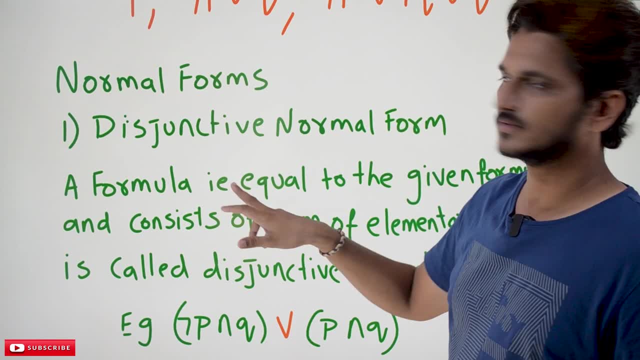 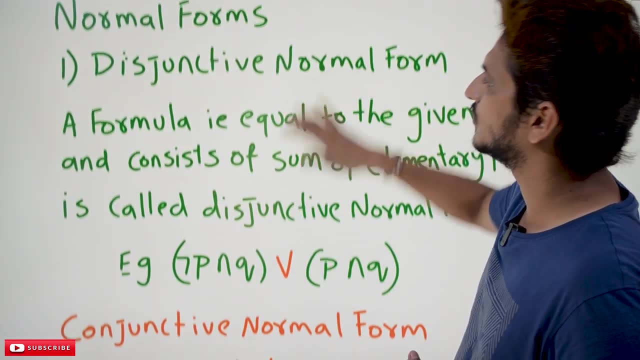 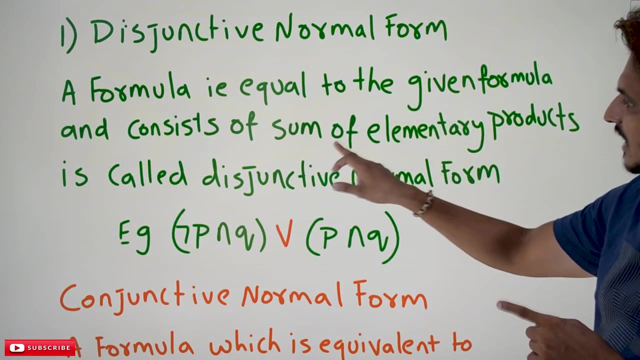 of normal forms. one is disjunct to normal forms. disjunct to normal form. second one is conjunct to normal form. here we are going to understand the definition of what's. disjunct to normal form means a formula that is equal to the given formula and consist of sum of elementary products. 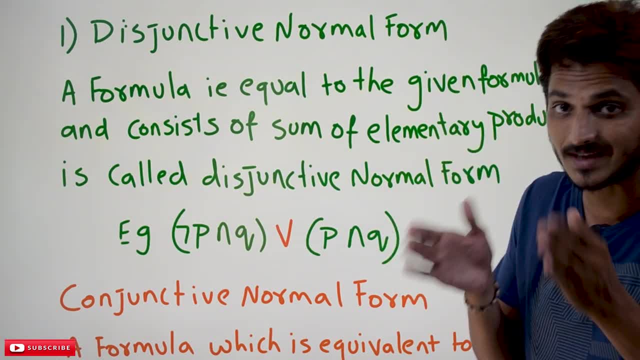 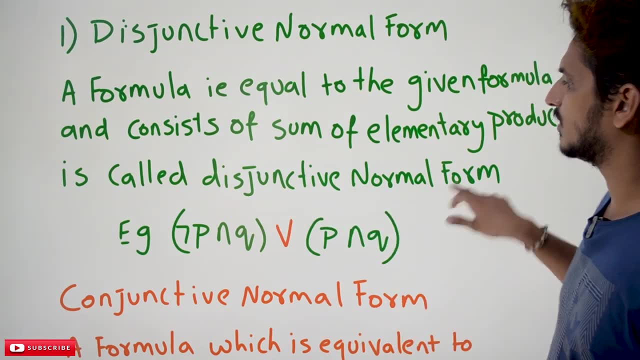 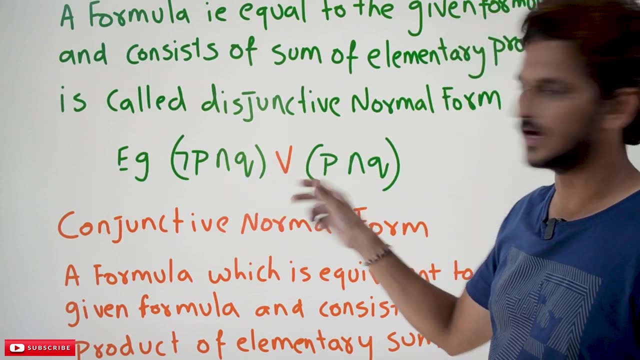 if your formula, if your proposition contains sum of elementary products, if it is in that form, we call it as a disjunct to normal form. disjunct to means disjunction. disjunction means sum, sum of elementary products. this simple proposition, we call it as elementary product. 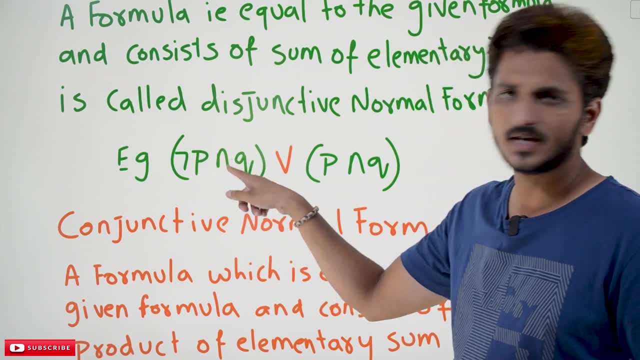 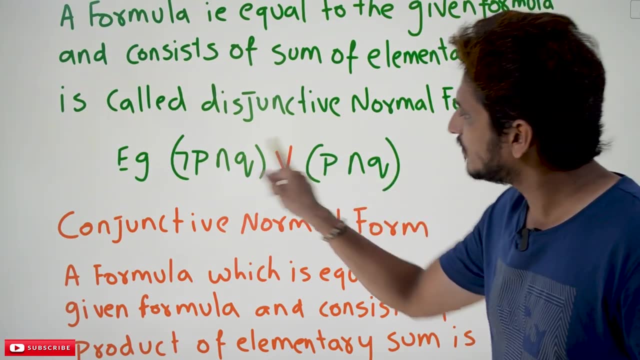 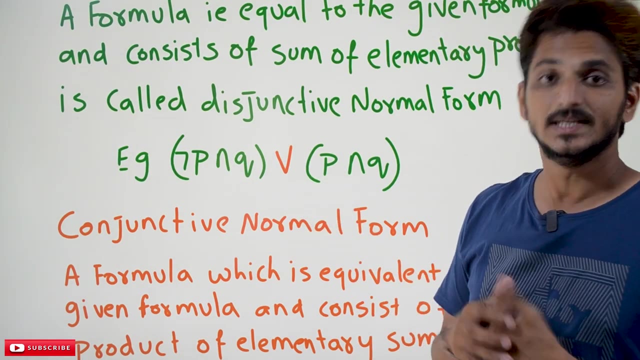 because it is in the form of a negation- p conjunction q. this we call it as elementary product- p conjunction q- sum of elementary products. if it is in this form, then we call it as disjunct to normal form, similarly conjunct to normal form. the next one is conjunct to normal form, a formula which is: 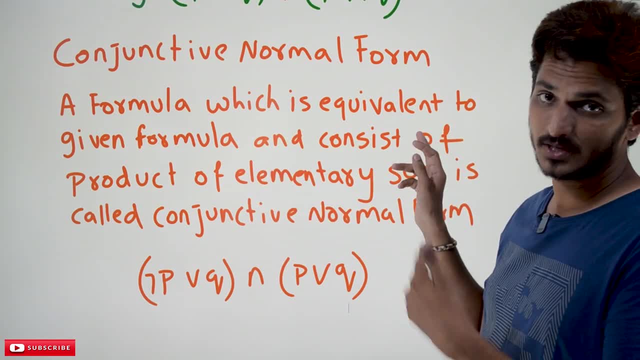 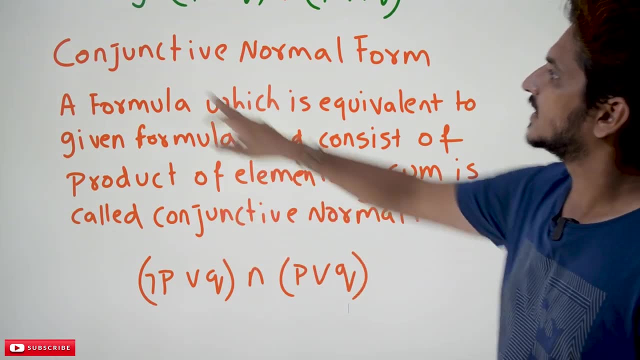 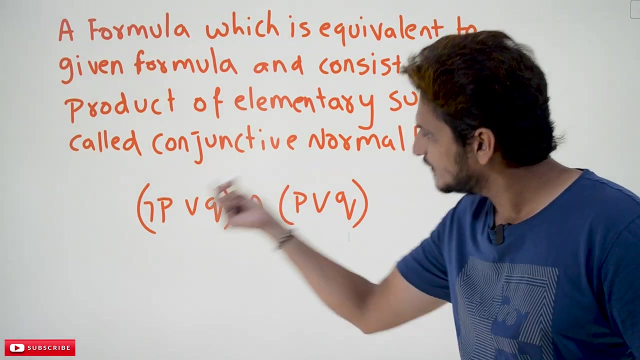 equivalent to the given formula and consist of, and it should be in the form of a product of elementary sums, is called as conjunct to normal form. conjunction means. conjunction means a product. product of elementary sum: see product of elementary sums. product of elementary sum. this proposition is in the form of elementary sum. 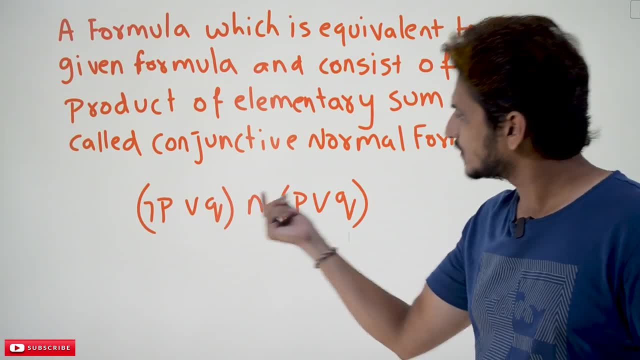 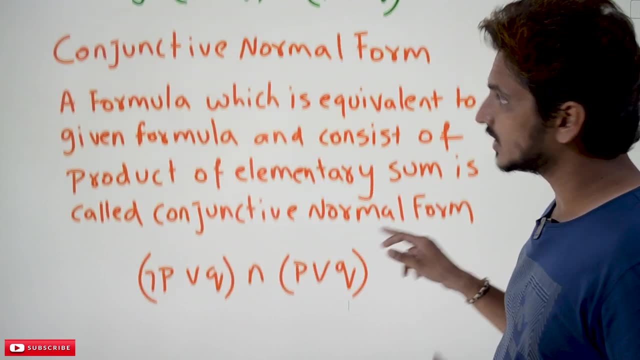 this proposition is in the form of elementary sum, so product of elementary sums. if it is in this form then we call it as conjunct to normal form. so in our next classes we are going to do some practice examples: how to convert the given proposition into disjunct to normal form and conjunct to normal form. 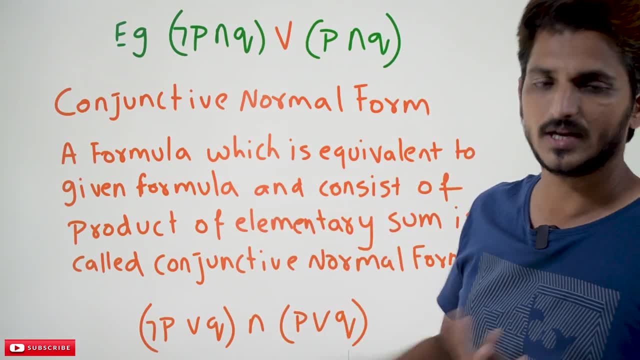 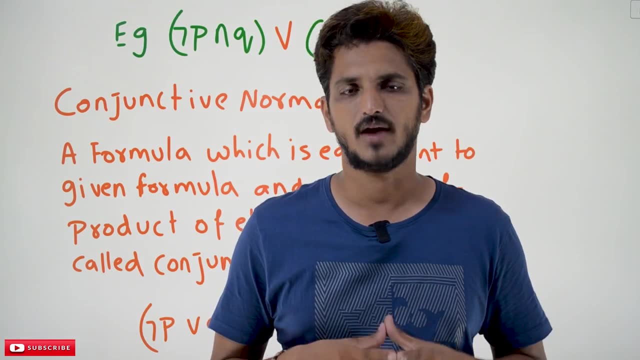 so these are the basics to understand in our next classes. hope you understand this class. if you have any questions regarding the concept, please post your questions in the comment section below. thanks for watching. if you haven't subscribed to our channel, please subscribe to our channel and we will see you in the next video. 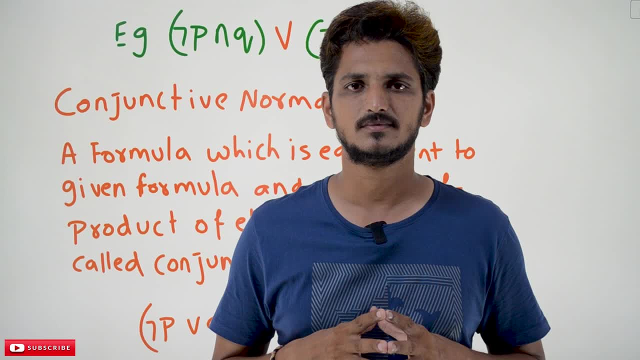 if you have not subscribed to our channel, please subscribe to our channel and press bell icon for the latest updates. thank you.